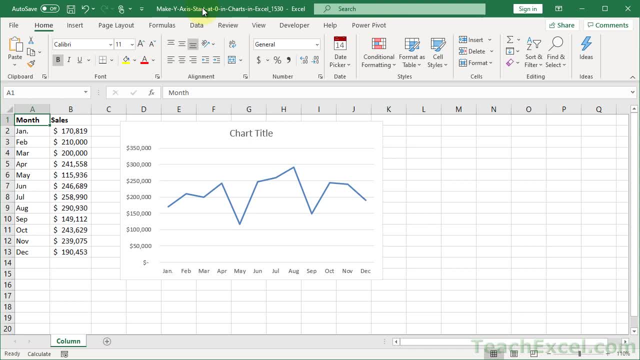 Here I'll show you how to make the Y or vertical axis start at whatever you want for charts in Excel, So it could start at 0, or start at 100,000, or a million or a billion, or end as well at whatever you want. 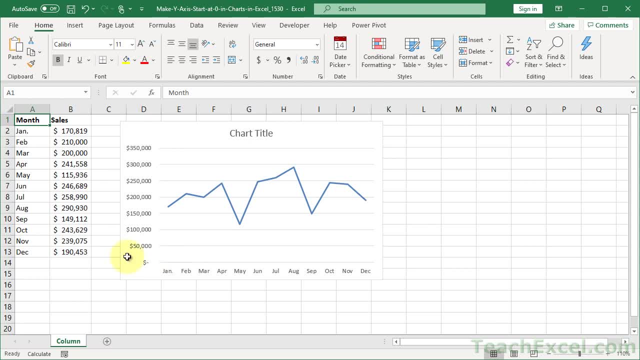 So I'm talking about this dude over here, and when you create charts automatically in Excel, it just kind of guesses what the bounds should be, But maybe that doesn't work for your data set or what you just want your chart to look like. 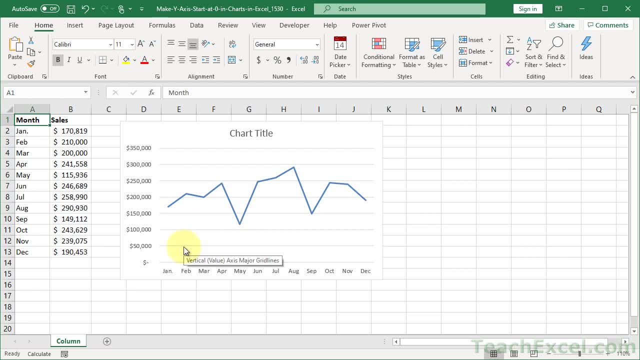 So insert your chart, All is good. Now let's go and edit it. First, we're going to click the chart and I'm going to show you a couple different ways to get to these options, because Excel loves to keep updating everything and changing where it's found. 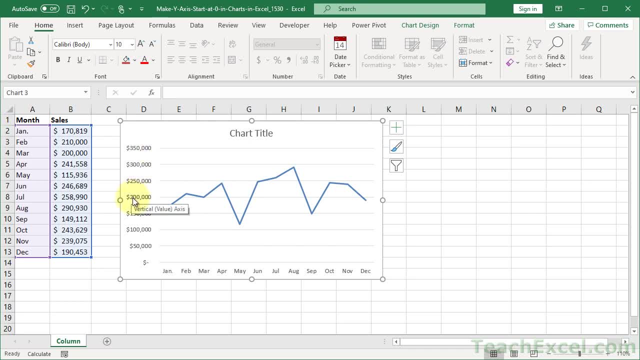 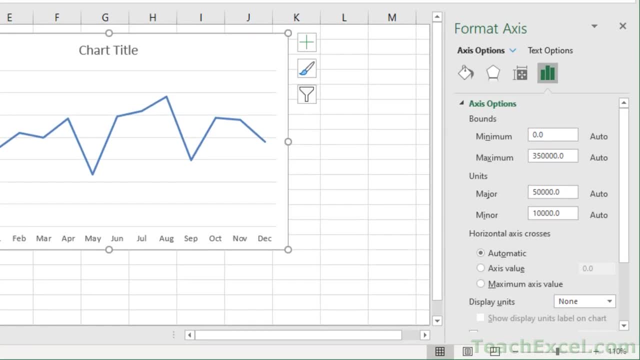 So we're in the chart. You want to change this? An amazing tip one of you showed me not that long ago: Just double-click the axis. Perfect. Now we are actually exactly where we want to be. So we have this little window over here and we have a bunch of different options. 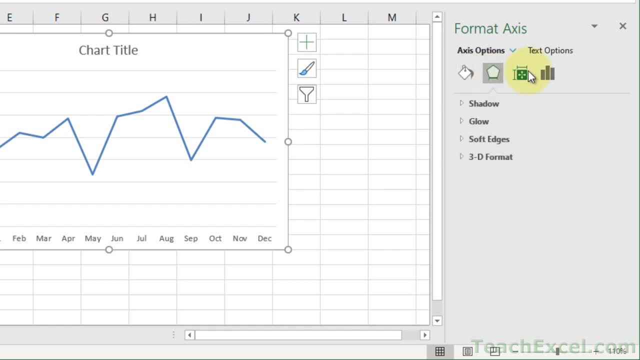 But sometimes you could be on the paint bucket or this dude or this dude, But what you want to do when you are in axis options, so make sure it's format: axis, axis options. and then we go to the little chart bar chart thing, which is also axis options. 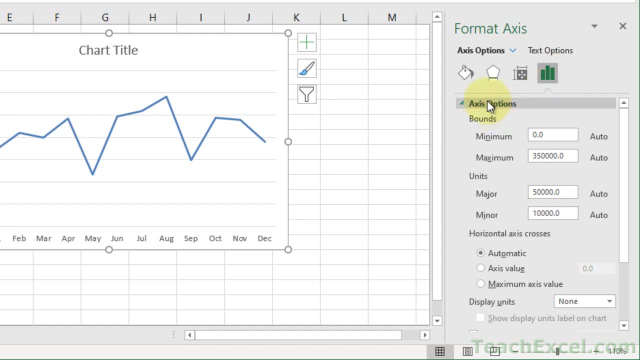 And then we go down here to another axis options, So it's like the third level of axis options, And then you go right here to bounds. You have a minimum and a maximum. So let's watch the chart when I change my minimum. 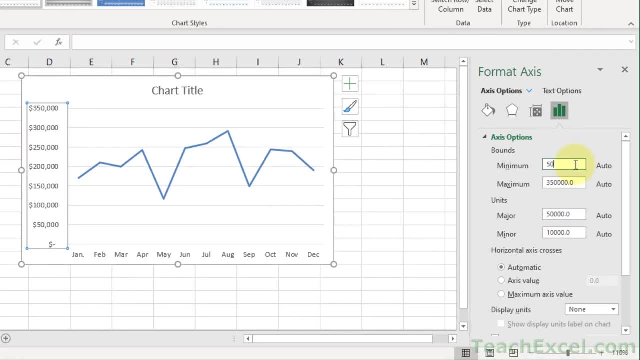 It's currently at zero. Let's say I want it to be 50,000. Awesome. And let's say I want to replace 350,000 with 300,000. Awesome. So the chart looks quite a bit different now. 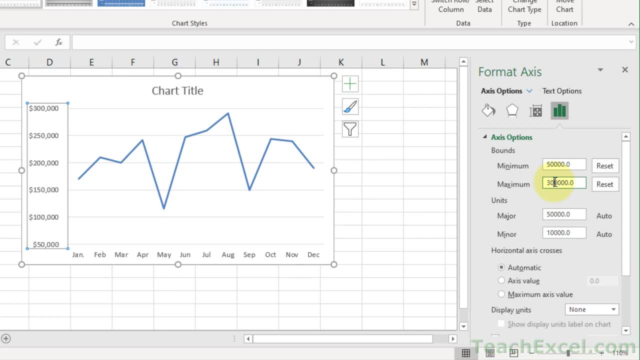 We've removed excess stuff or space. If you want, just go ahead and click reset and it will send you back to the default. So you see auto here. That means Excel has tried to guess how you want to display it, what you want the bounds to be.